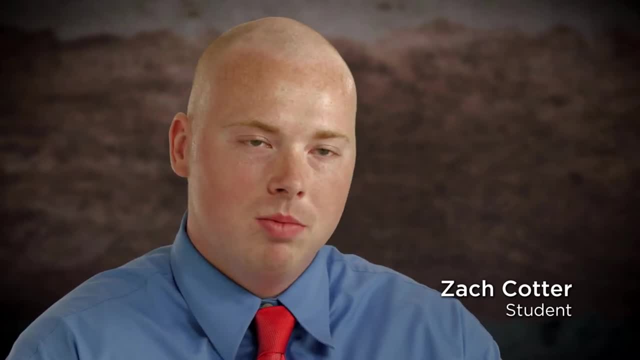 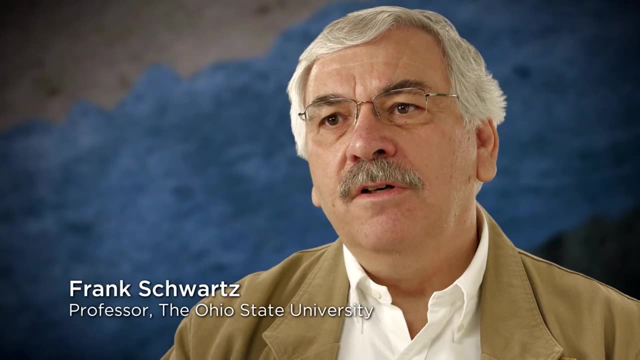 It just rained when I took a geology class and that sparked my interest And from that class on I knew what I wanted to do. These days, when students are coming to college, you see that they're really interested in different paths. 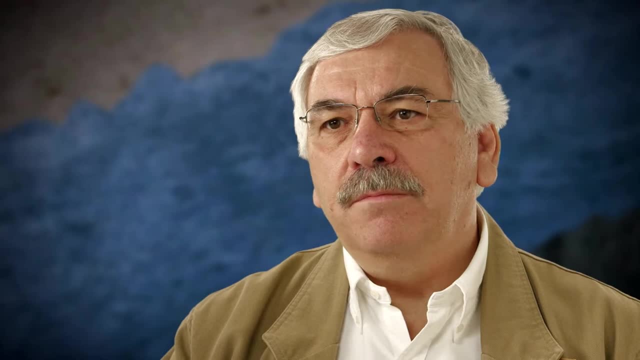 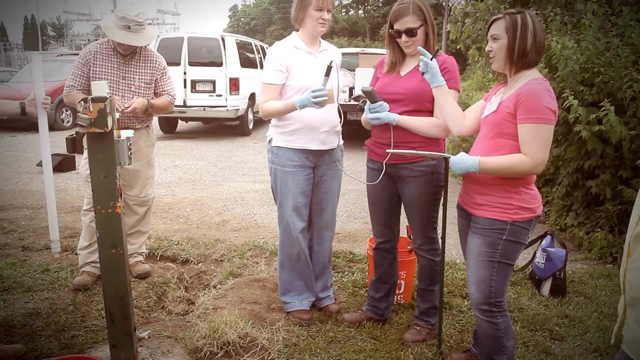 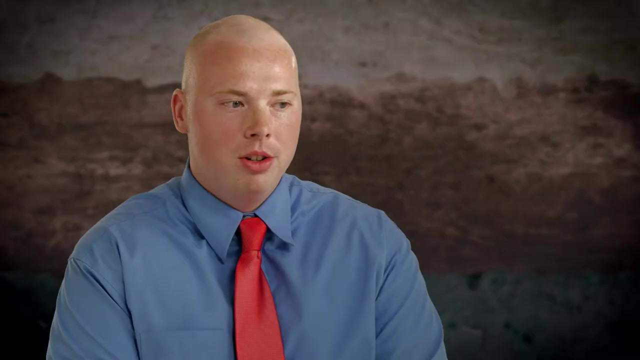 I mean, many start out in engineering or even in arts and they end up taking an introductory geology course, for example, and they really find that attractive. If you get into this field, you can really specialize in anything You can do with resource management. You can do with just studying groundwater saltwater interactions. 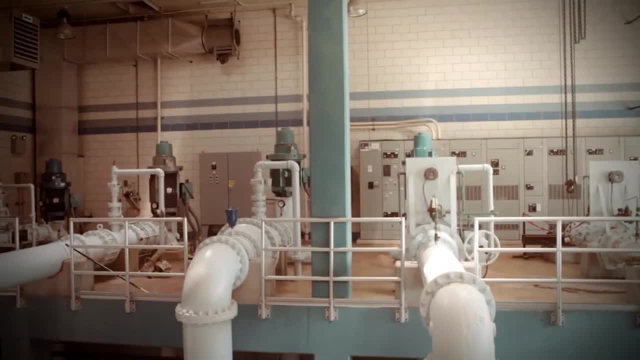 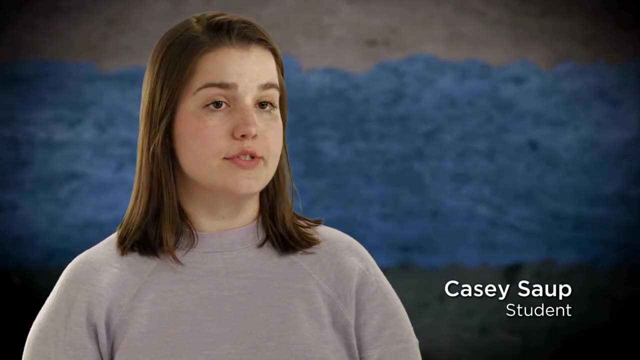 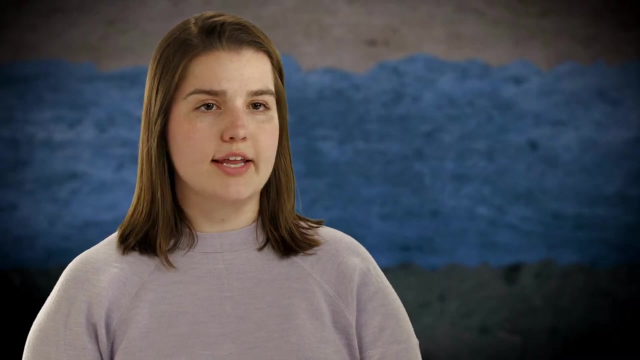 I mean water supply remediation, freshwater distribution, geology, hydrogeology. I took geochemistry and geomicrobiology And in geochemistry that was the first course I took And we briefly touched on the arsenic contamination in groundwater in Asia and that kind of piqued my interest. 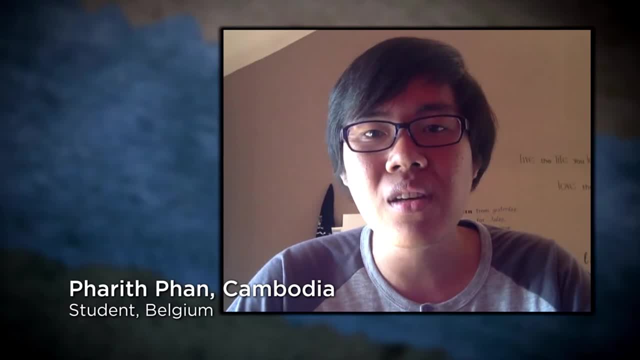 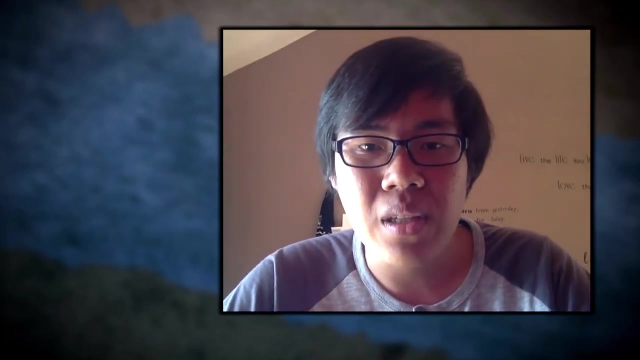 In my country there's just a few people that are concerned about the groundwater because we have a lot of surface water, So people are concerned only about the surface water. So I want to study about the groundwater and I can develop. I love it in my country as well. 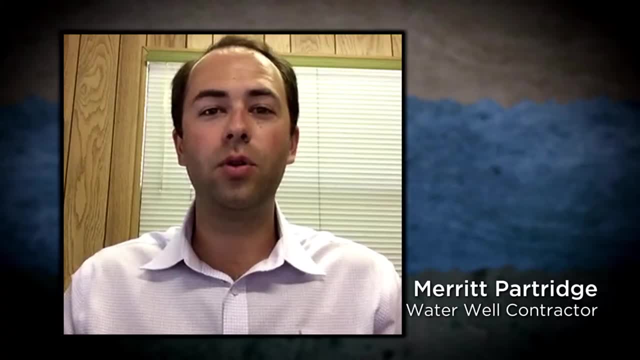 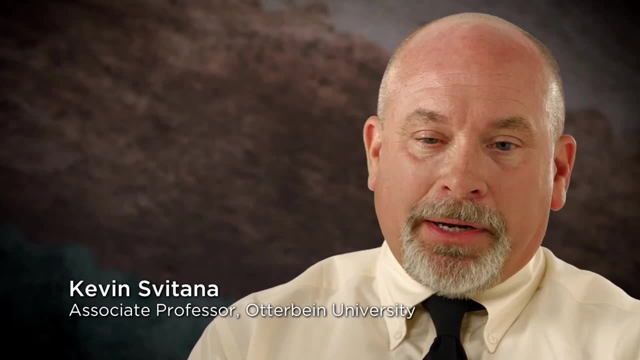 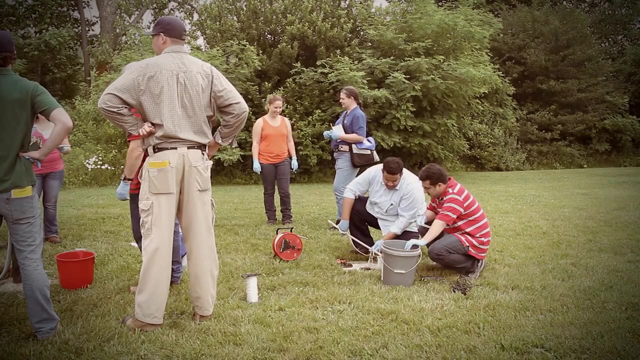 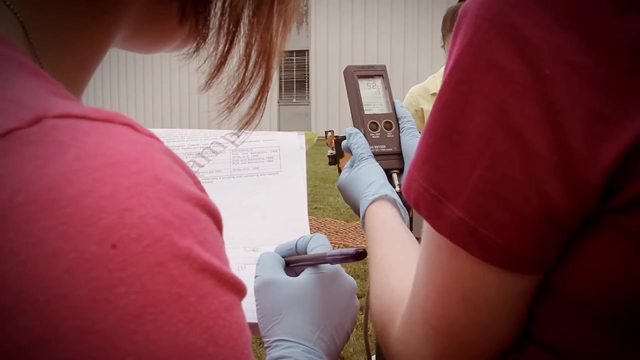 Providing groundwater to people is a very rewarding career. When I drill a well, I know I've done something good for somebody. A lot of what groundwater scientists do is try to make water quality better and try to understand water systems too, And I think that's kind of rewarding when you can work with people and think about how what you're doing is part of a larger system and how you fit into that piece of the system. 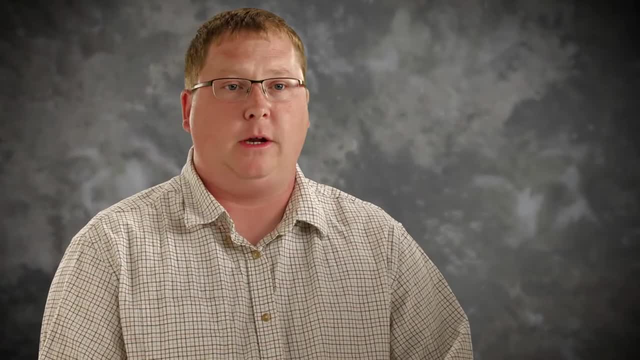 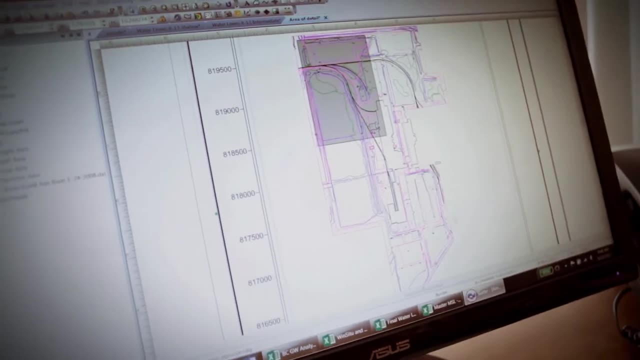 Everything I've done before was It's completely money-driven and nothing concerned about taking care of the environment. so I wanted to do something. on the other end, I want to make an impact in the scientific world, but I really want to affect the general public. 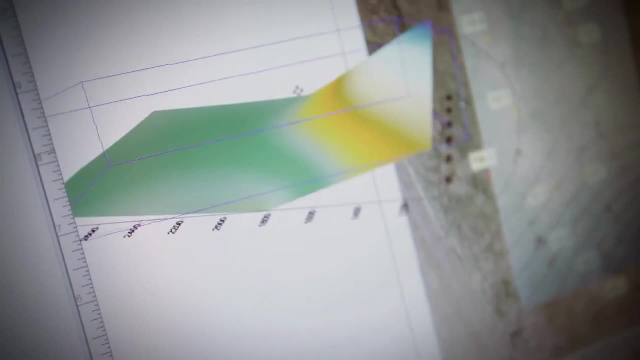 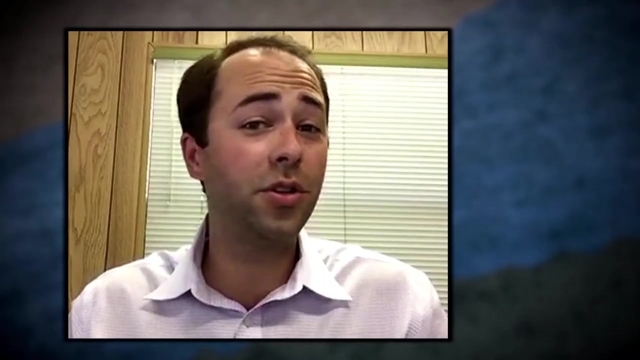 I saw a big opportunity there to make sure that people have the freshwater resources that they need. There are many places in the world where you just cannot live without groundwater, and when I drill a water well, I'm providing a lifeline to somebody. 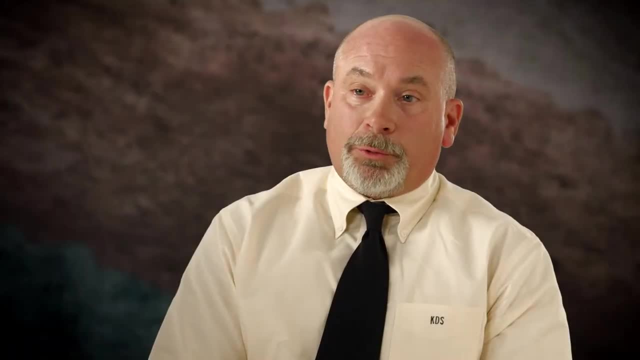 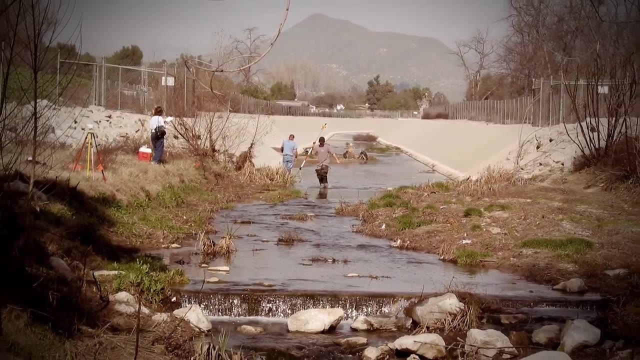 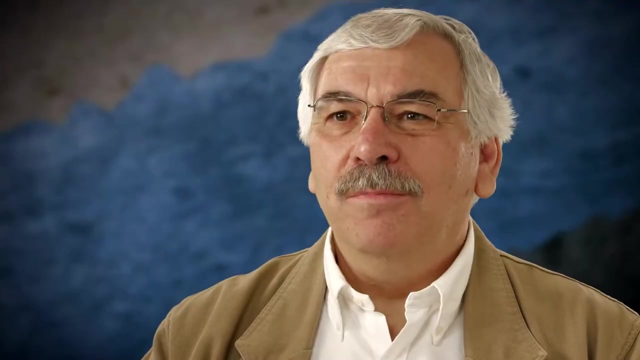 I think people are starting to realize that water management is truly a challenging career and there's more and more of a demand for it. I want to be a problem solver and part of the solution, not part of the problem. There's lots of places in college you can go to get a degree, but there's not so many places in college you can go to get a job. 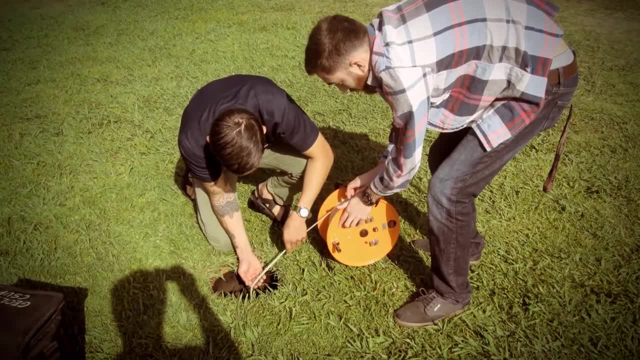 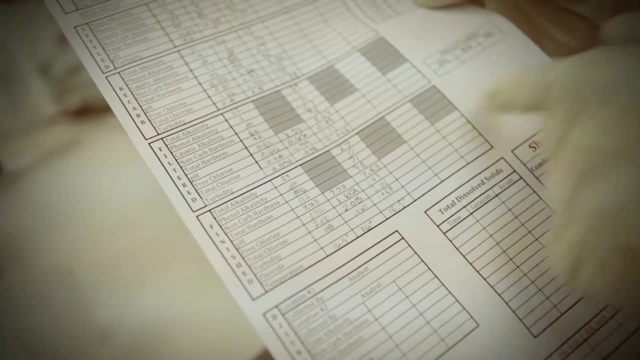 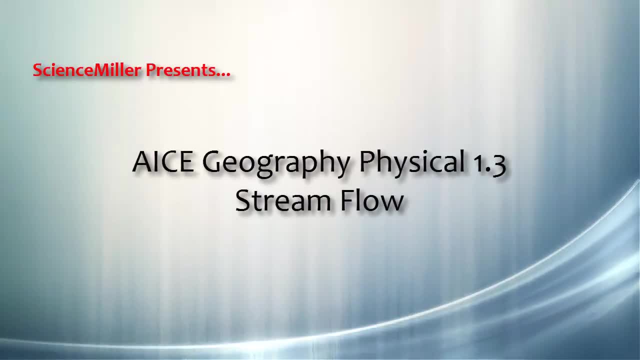 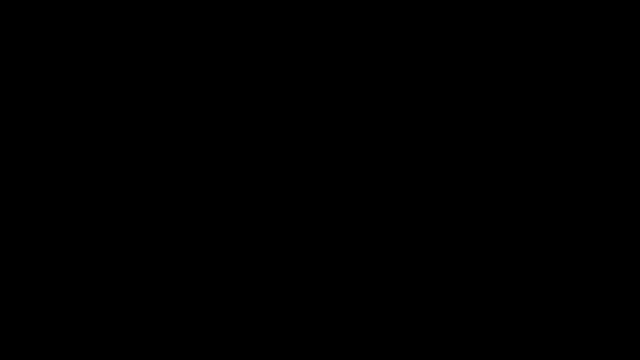 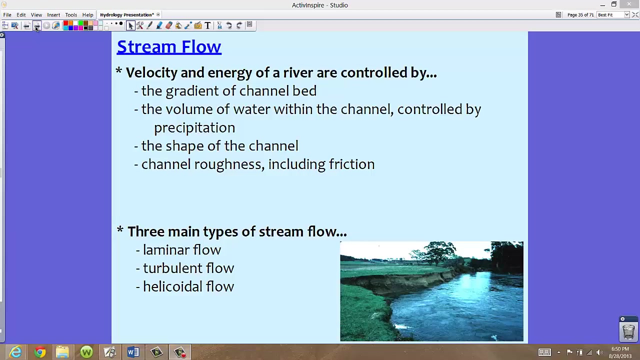 Now we've talked about transport, deposition and erosion. Let's talk about the stream flow, the actual movement of the river, because this is extremely important. You're going to see different types of flow in streams and that's going to cause different sorts of landforms forming. 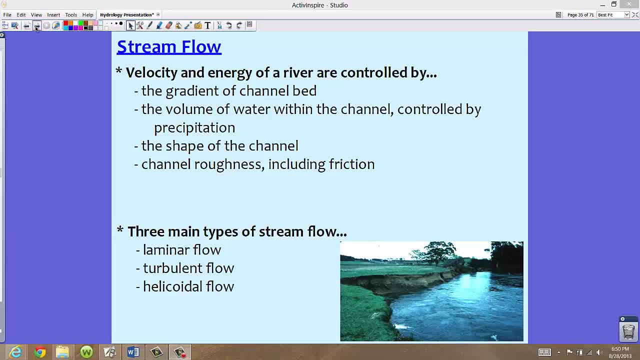 on each side of the bank or around the general area. So it's very important to understand that the velocity and the energy of a river are controlled by several factors. Now, starting off, this factor is the gradient of the channel bed, the slope, basically how steep it is. 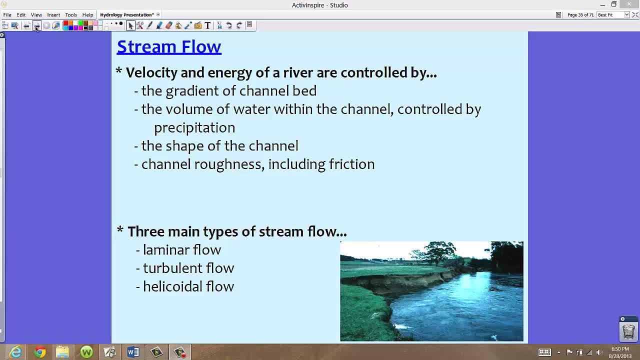 the volume of the water within the channel, which is usually controlled by precipitation, so the amount of water in the channel, the shape of the channel- remember, not all channel shapes are kind of like bowls, Some of them are like rectangular, some of them might be square.